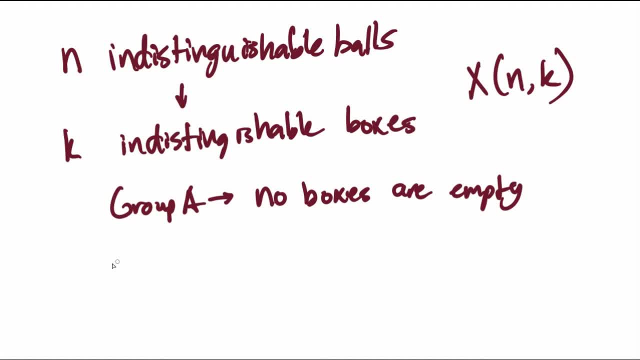 And let's actually. And the second group, of course, is that there is at least one empty box. But let's approach group A first. Let's see if we can actually subdivide this question. So first, assuming no boxes are empty, how many ways can we put an indistinguishable ball into? 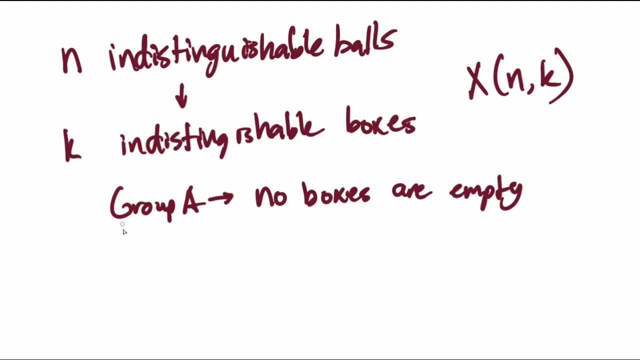 Okay, non-empty, indistinguishable boxes, And there's actually a notation for this. It's the way you partition n into k boxes And the partition indicates that none of the boxes are empty. And the formula for this is that there is no easy formula because it's a recurrence relation. 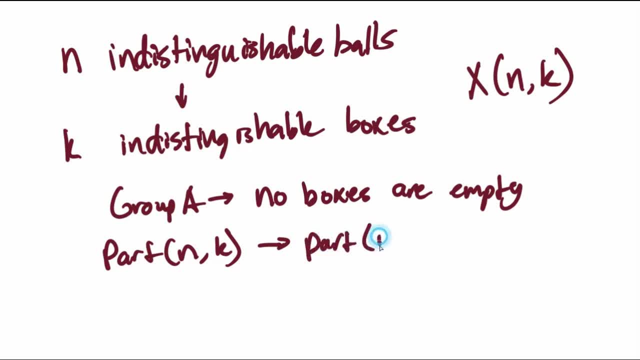 So actually it would look like this: All right, So what does this mean? right? So the number of ways to partition n indistinguishable balls into k indistinguishable boxes- assuming no box is empty- is the number of ways to partition n-1 indistinguishable balls into k-1 non-empty indistinguishable boxes. 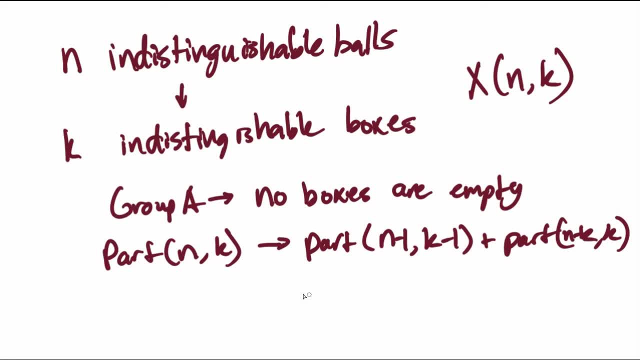 plus n-k. indistinguishable balls into k-1 non-empty indistinguishable boxes. And how do we? Why is this true? Let's prove this. So say: you've got n balls. right, You've got n balls and you've got to put them into k non-empty, indistinguishable boxes. 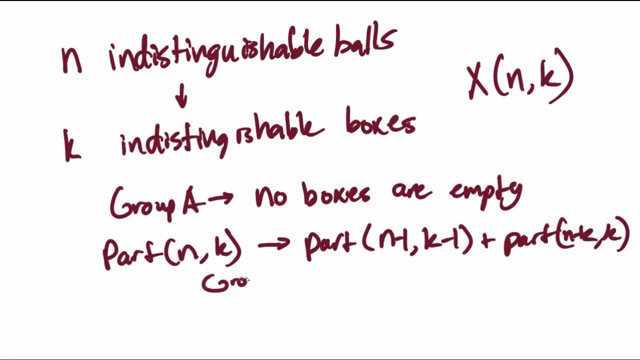 There are two ways you can group this. So group- Let's do lowercase a- is where at least one box has exactly one ball. So the numbers in this group would be something like one comma, something one comma. dot, dot, dot, dot dot. 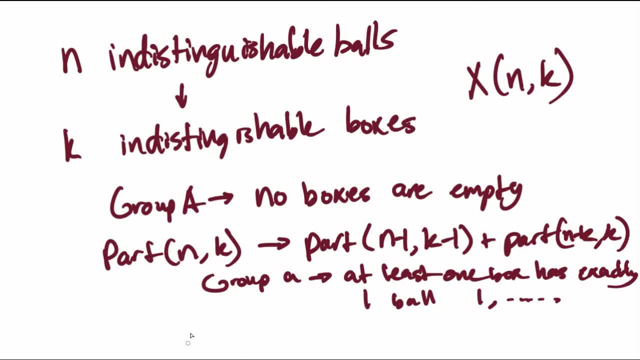 So at least one box has exactly one ball And group b is all boxes have at least two balls. And let's see if we can match the groups to the parts of this equation. Every single combination under the partition of n comma k has to fit under one of these groups. 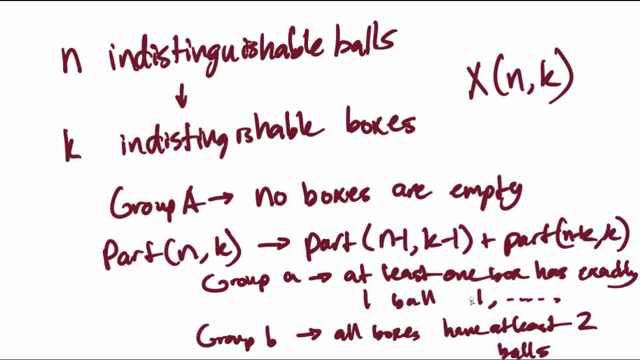 Either the combination has at least one box has exactly one ball, or all the boxes have at least two balls. So for every combination these are disjoint distinct groups that make up partition n-k, Because a combination has to go under one of these groups. 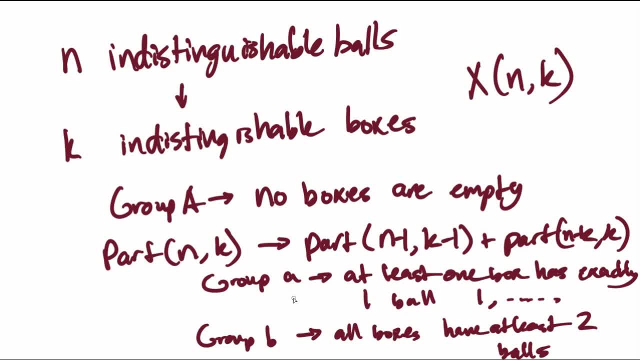 and they cannot be in both groups. So actually the number of combinations in group a corresponds to the number of partitions in n-1 indistinguishable balls and k-1 indistinguishable boxes. Why is this? Because, let's say, you take away that one box with exactly one ball. 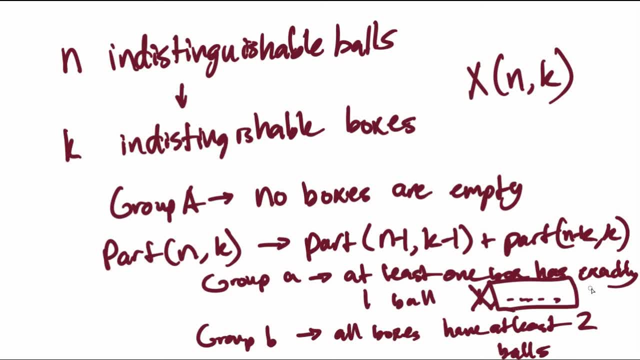 And then over here you can organize the rest of the balls in n-1, the rest of the n-1 balls in k-1 boxes. So essentially you take away one of the boxes with at least exactly one ball in it. 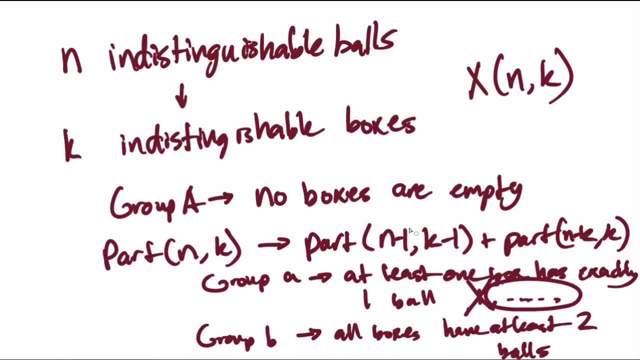 And then the number of ways to organize the rest of them is there are n-1 balls in k-1 boxes, so it's partition n-1 k-1.. The other scenario is if all boxes have at least two balls. 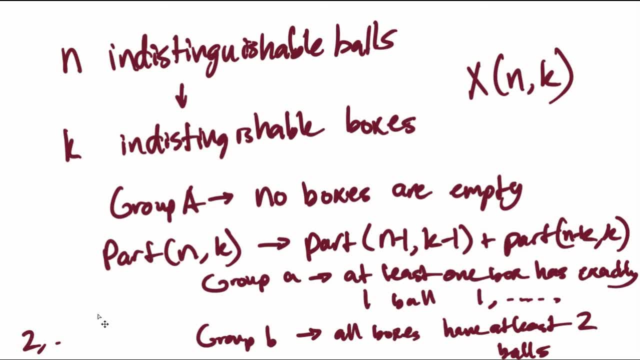 So that will go like two In this case, because you know that all the boxes have at least two balls you can actually subtract. you can actually subtract a ball from every single box. So if you subtract a ball from all k boxes, 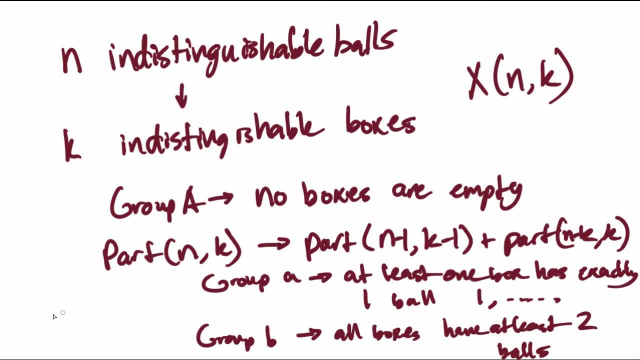 you'll end up with. you'll end up with n-k balls and they're divided into k boxes And that's partition n-k k. For every single combination in which you can subdivide n-k balls into k boxes, you can add one to each one of those combinations. 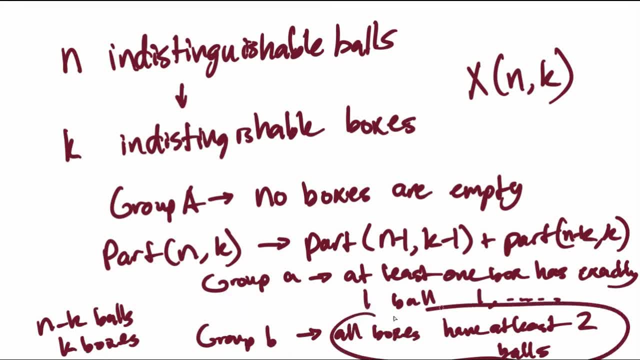 to get a combination in group B where all the boxes have at least two balls. It's a bijection. So that basically proves it. The number of ways that all boxes have at least two balls is equal to partition of n-k indistinguishable balls in k indistinguishable boxes. 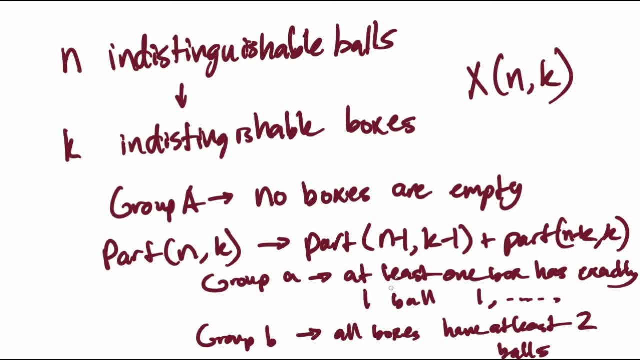 and in the group where at least one box has exactly one ball. take away that box. you get a number of partitions of n-1 into k-1 boxes And both of those make up the number of ways to partition n-1 and indistinguishable balls. 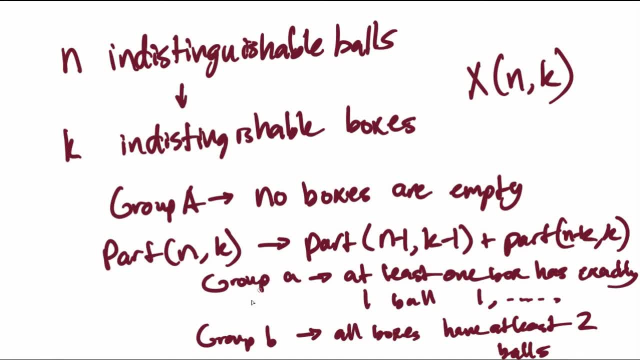 into k non-empty, indistinguishable boxes. Phew, So we have that. We have that useful equation, And there really isn't an easy way to simplify this into a formula. So actually, if there's no way to simplify this into a formula, 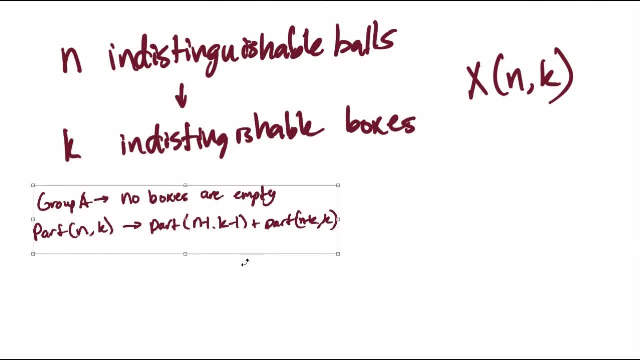 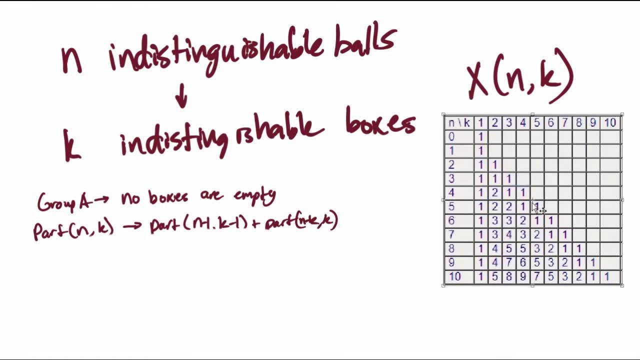 we gotta just bash it out. And when I say bash it out, I mean I have the table right here of partition partitions. So partitions and k. So there's the table, So, as you can see, the number of ways to partition. 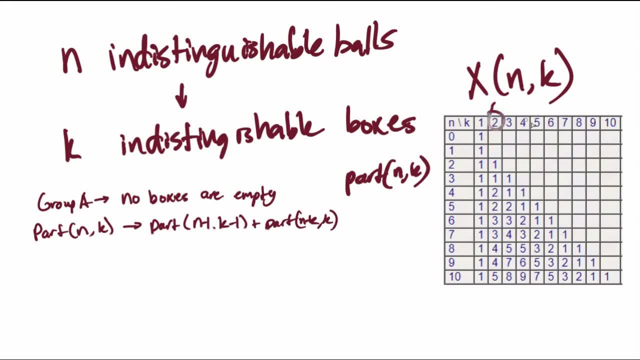 nine indistinguishable balls into two non-empty indistinguishable boxes would be four. Make sense. Okay, So we have this useful table here, But we only have group A down. The other group B is where at least one box is empty. 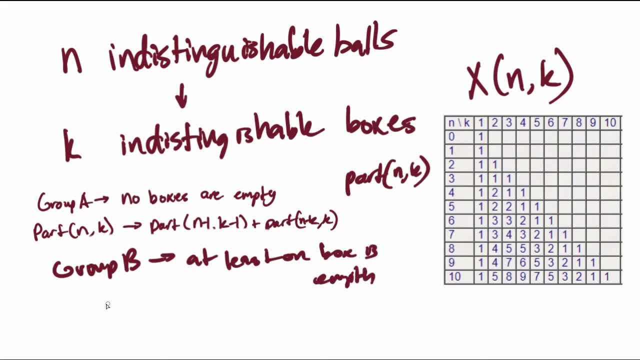 And then we do the same thing we did for group lowercase a. So if it's the zero, something, something, something, we take away that zero And what's left over is: we have, we have n balls, n indistinguishable balls, because we didn't take away any balls. 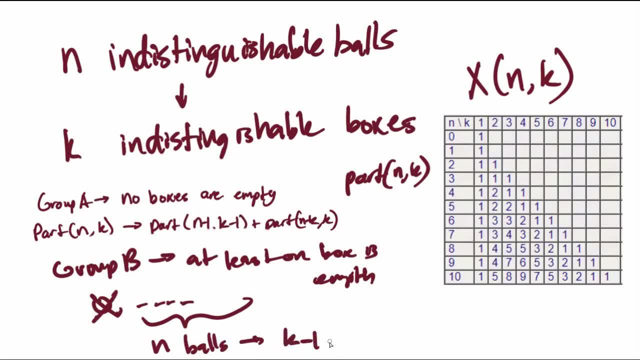 into k minus one indistinguishable boxes. So the number of ways in group B is actually x and k minus one. Alright, Seems pretty good, Pretty, pretty, pretty good, Alright. So actually we now have this neat little formula. 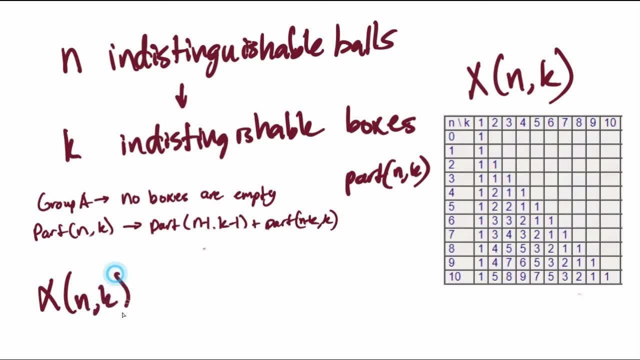 So now we have that x and k is equal to partition n- k plus x, n k minus one, And we know that x and k minus one is equal to partition n- k minus one plus x- n k minus two, And hopefully you know where I'm going with this. 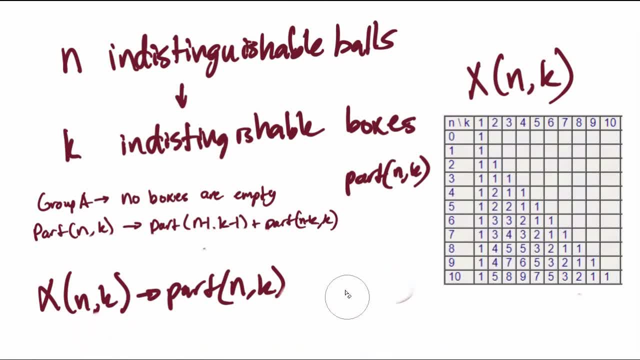 Is that all of this actually simplifies And you can actually do partition n k minus one plus partition n k minus two plus partition n k minus three, dot, dot, dot all the way to partition n one, which this part is equal to one. So actually, 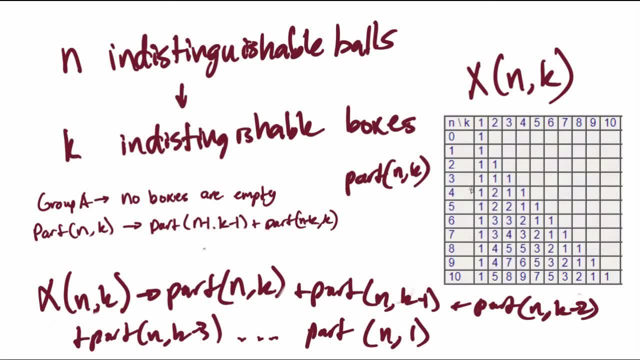 So if you want to find ways to put n indistinguishable balls into three indistinguishable boxes- assuming they are they can be non-empty- then you would actually just add up all the numbers behind it and that number in that cell. So to illustrate this, 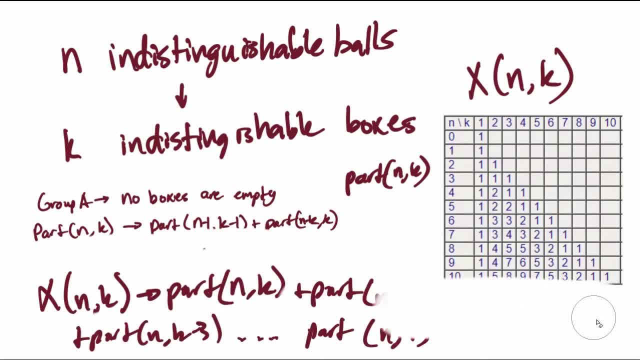 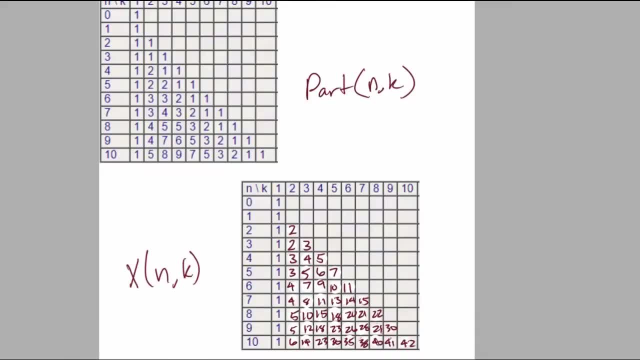 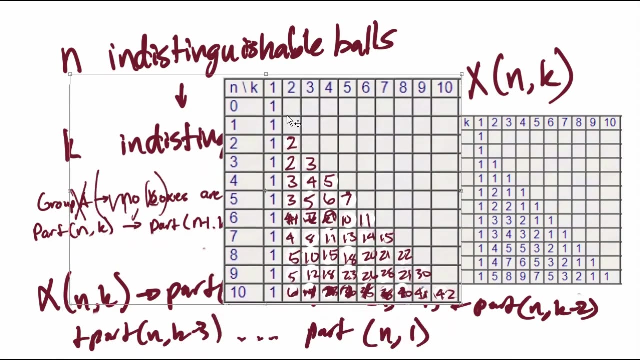 I put together a table of my own, so to speak. I'll just shift over. So this is a table of my own. I'm not sure if you can see it, So I'll copy it over. Oh look, It's sort of transparent. 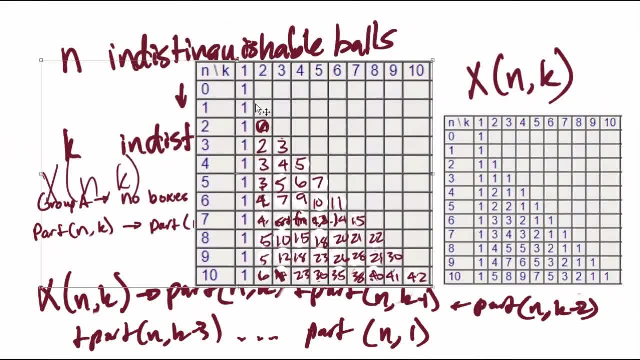 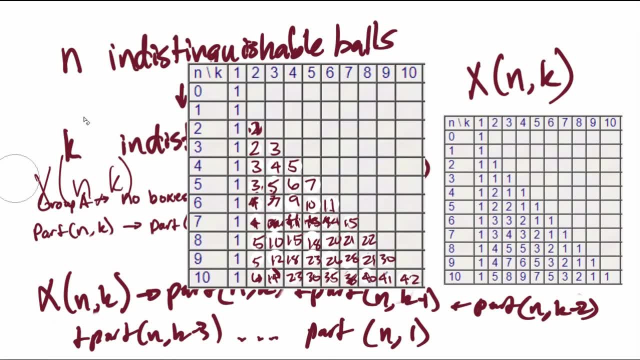 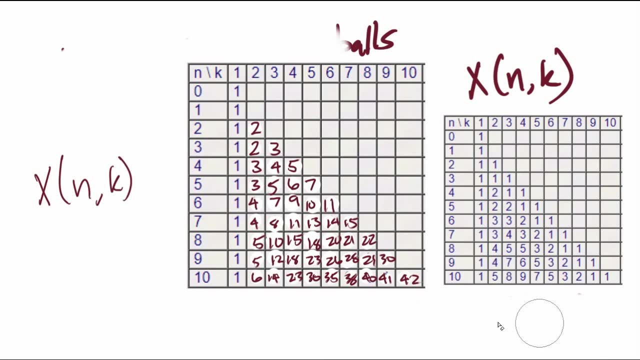 That's a tad annoying. Let me just. Let me just erase everything under it. So if you actually compare this table to that table, So this table is, This table is of. This table is of x. The number of ways to put n indistinguishable balls. 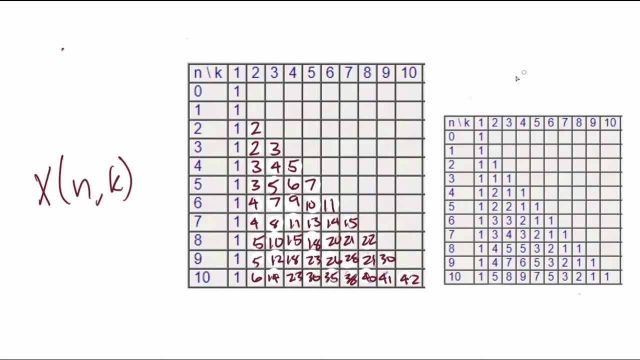 into k indistinguishable boxes, Assuming the boxes can be empty, And this is the ways to partition them. And if we compare the two graphs, we can see that this 4 right here is sort of the summation of these three cells, And this 11 right here,